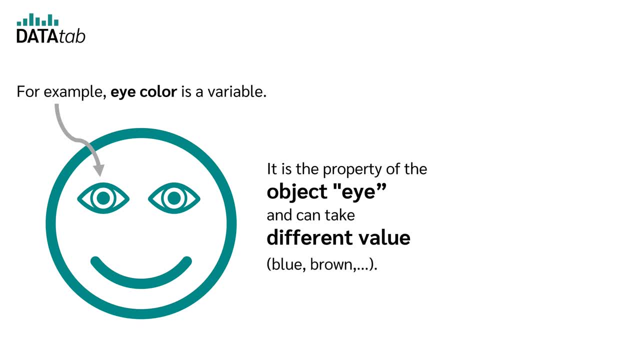 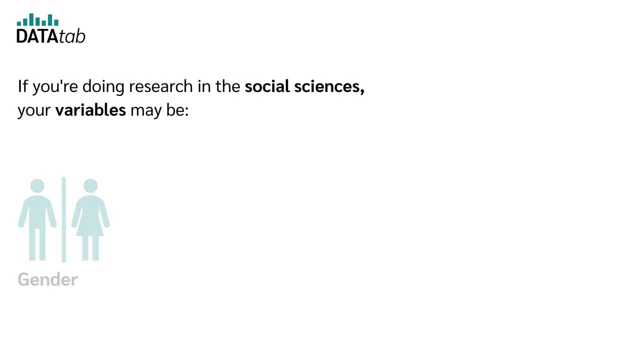 and can take different values, for example, blue, brown and so on and so forth. If you're doing research in the social sciences, your variables may be gender, income or attitude towards environmental protection. If you're doing research in the medical field, your variables may 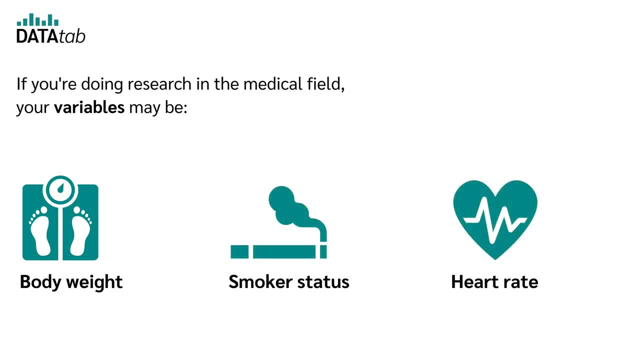 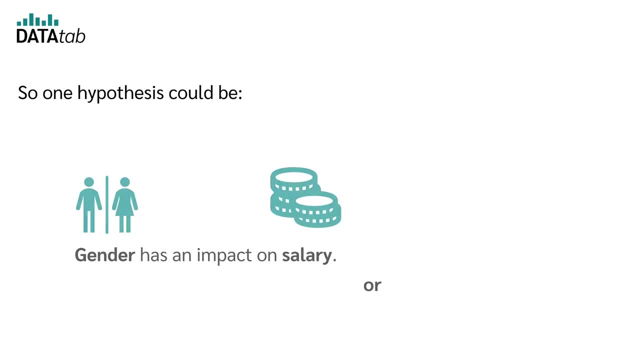 be body weight, smoker status, heart rate. So one hypothesis could be: gender has an impact on salary, Or there is a correlation between body weight and heart rate. But what is it about null and alternative hypotheses? Two hypotheses are always formulated that assert the opposite. These are called the null and alternative hypotheses. The null hypothesis. 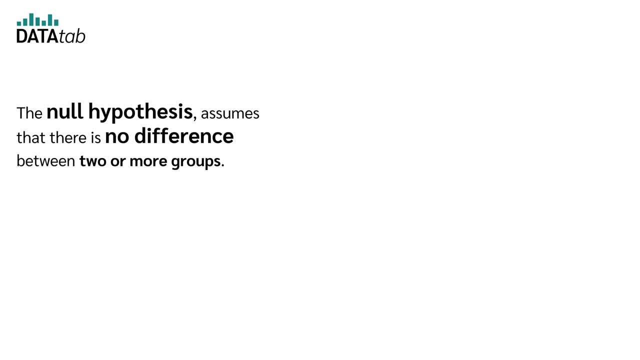 assumes that there is no difference between two or more groups. An example: the salary of women and men. The salary of men and women does not differ in Germany. In contrast, the alternative hypothesis assumes that there is a difference. Example: the salary of men and women does differ in Germany. 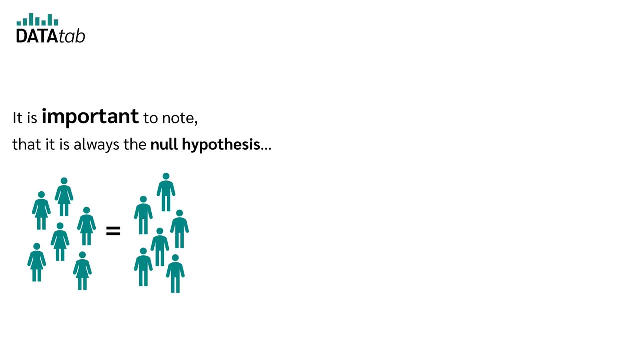 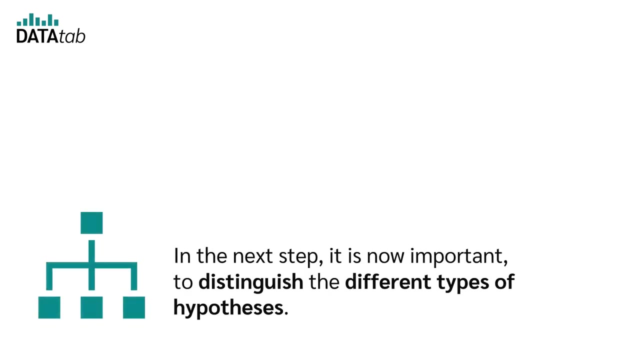 It is important to note that it is always the null hypothesis that is tested with a hypothesis test. Thus, the null hypothesis is always either rejected or not rejected. Learn more in our hypothesis test. In the next step, it is now important to distinguish the different types of hypotheses. 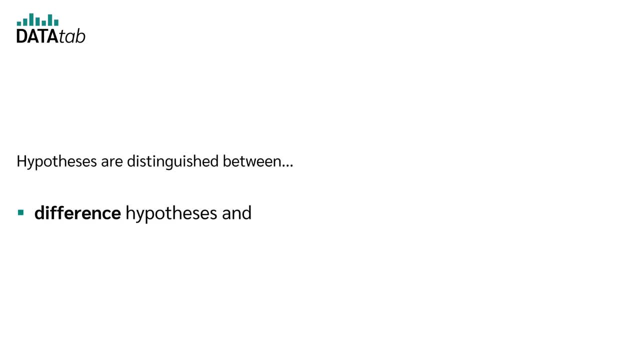 Hypotheses are distinguished between difference hypotheses and association hypotheses, as well as directed and undirected hypotheses. Let's start with difference and association hypotheses. Difference hypotheses test whether there is a difference between groups. Example: the salary of women and men does not differ in Germany. In contrast, the salary of men and women does not differ in Germany. 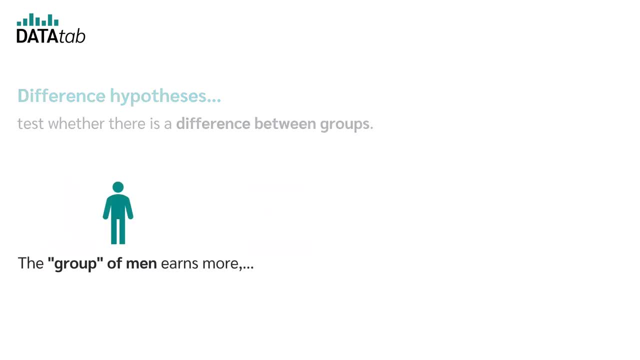 Example: the salary of men and women does not differ in Germany. In contrast, the salary of women and women does not differ in Germany. Example: the type of smoking is different between two groups. example: the group of men earns more than the group of women. 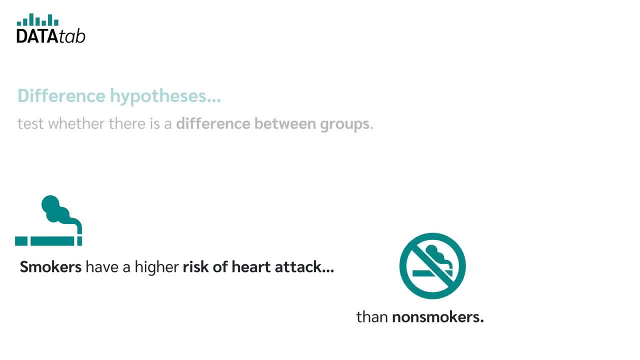 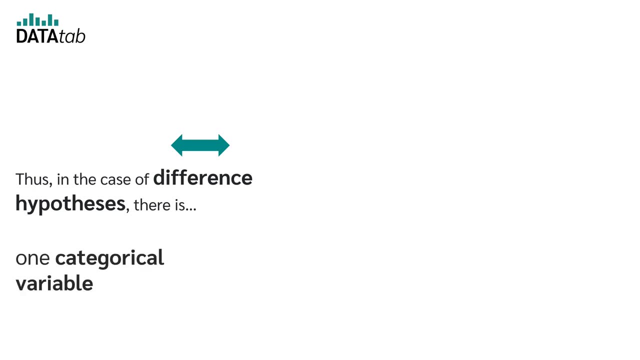 Smokers have a higher risk of heart attack than nonsmokers. Thus, in the case of differences hypotheses, there is one categorical variable and one ordinal or metric variable, NG8. The categorical variable is, for example, gender, with male and female, or smoking status, with smoking virginity.